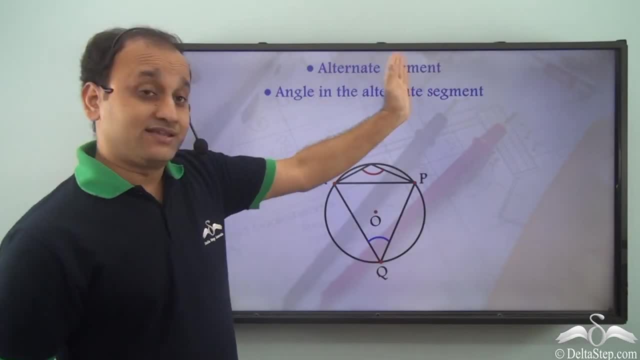 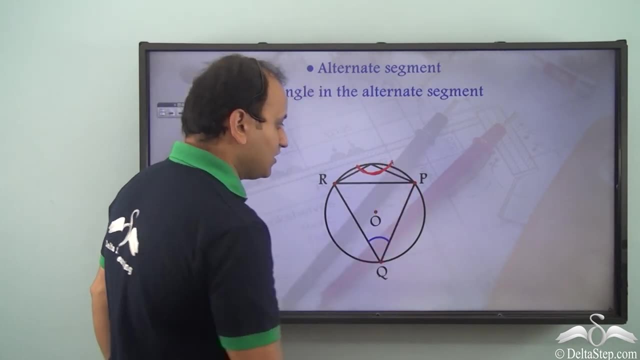 segments. let's discuss about angle in the alternate segment. Now, in this case, what do we see? Well, we have this particular angle which lies in this particular segment, isn't it? And if we talk about this angle, this lies in this. 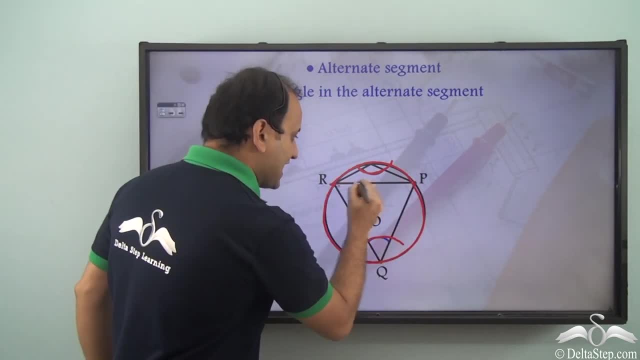 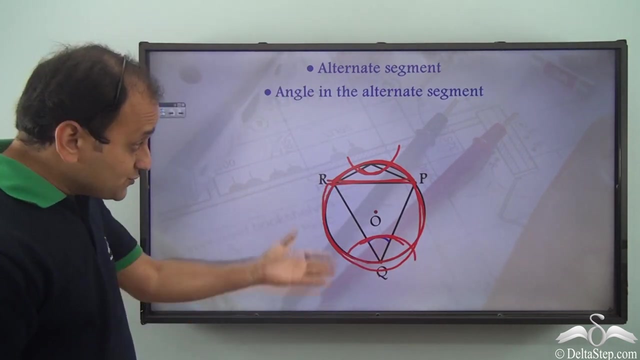 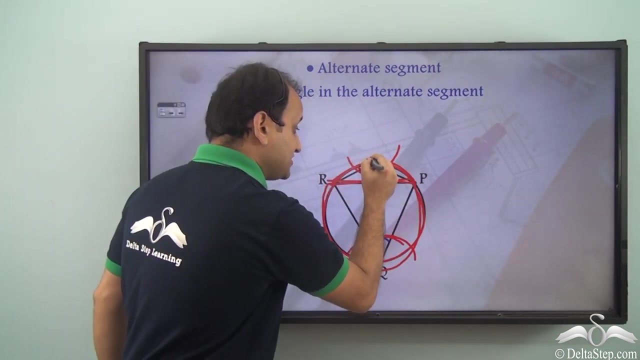 this particular segment, isn't it? You can clearly see that you have this area and you have this particular area. So one angle lies in this, other lies in the alternate segment. So we can say that angle PQR, and if I take a point here and name it, 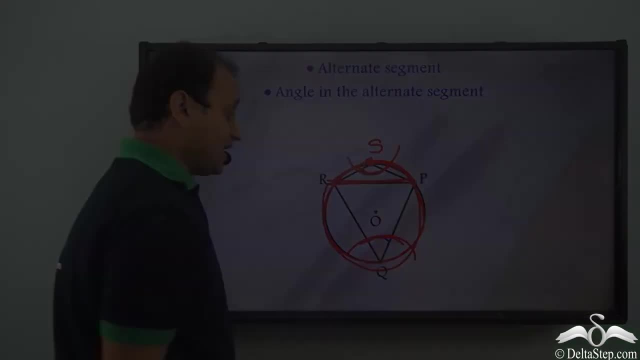 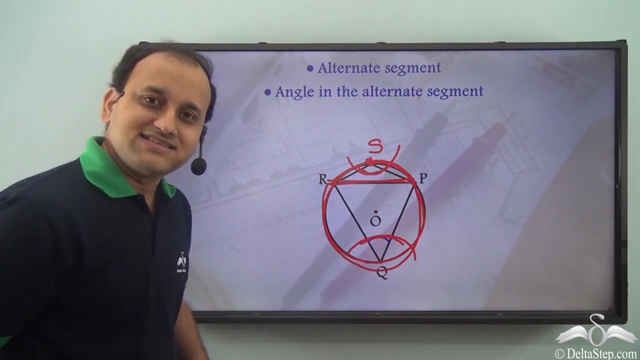 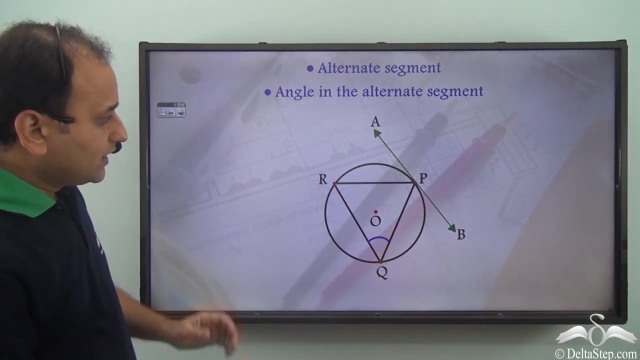 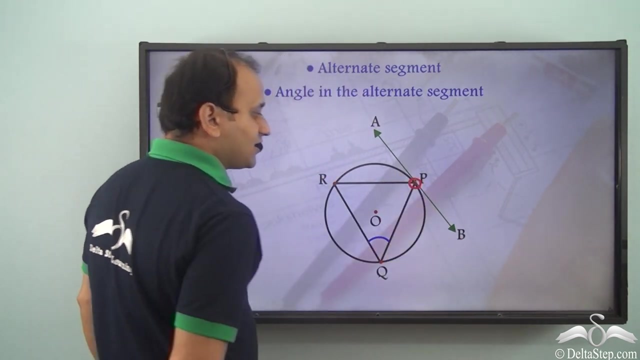 S, then angle RSP lie in alternate segments, or we can say that these are angles in alternate segments. So this is another important concept. Now, if we have a line that touches the circle exactly at this particular point, that is one end of the chord. 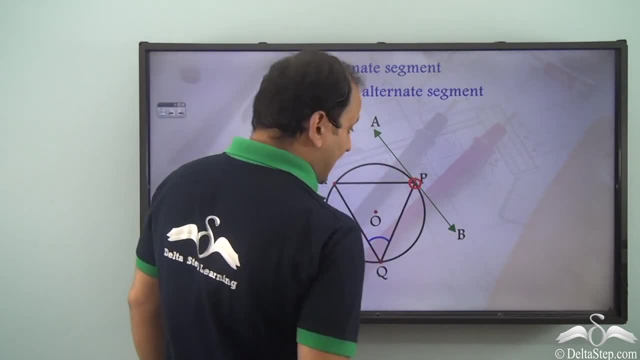 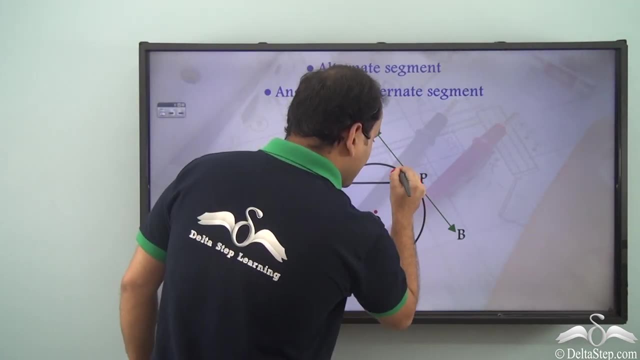 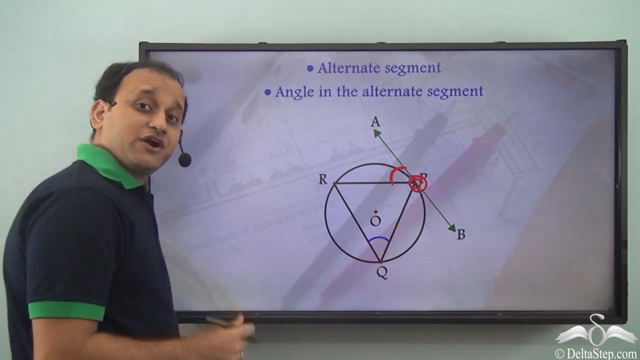 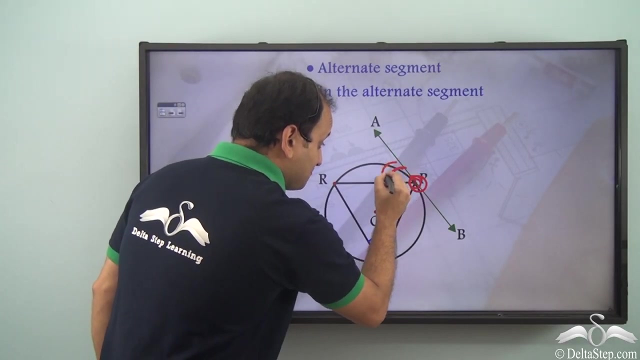 then what happens? Well, this gives rise to a very important theorem. So the theorem states that if you have this particular angle, which is being made by this line which touches the circle at this particular point P, which is one end of a chord, So this line, 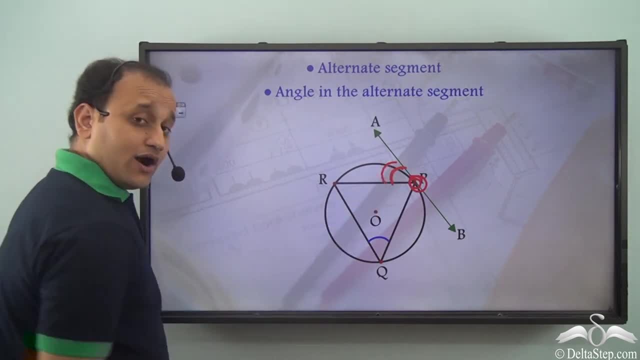 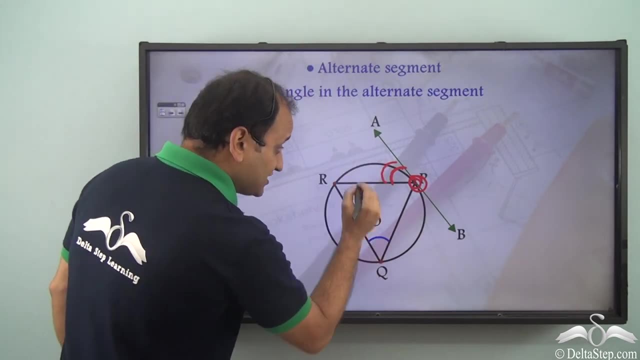 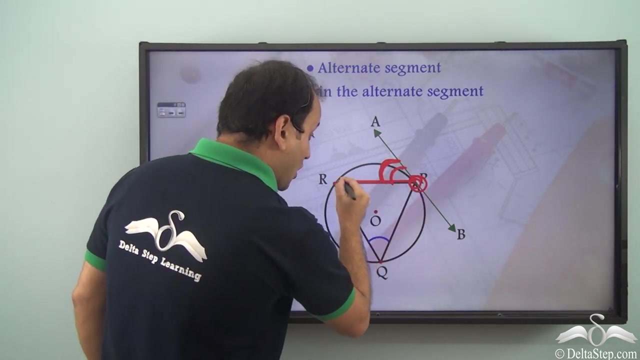 makes this particular angle with the chord RP. Now, the theorem which we are going to discuss states the relationship between this particular angle and the angle made by this particular chord in the alternate segment. So you can see that this angle is being made in this particular segment. right, It touches this particular segment. 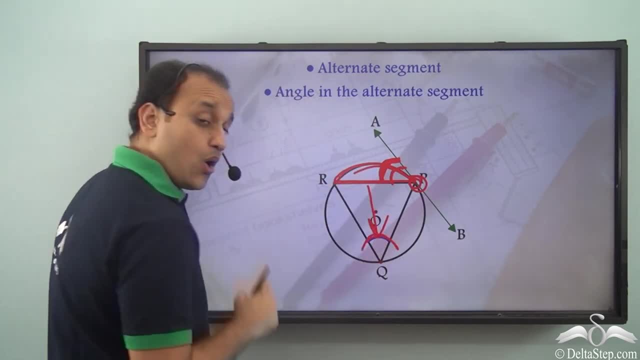 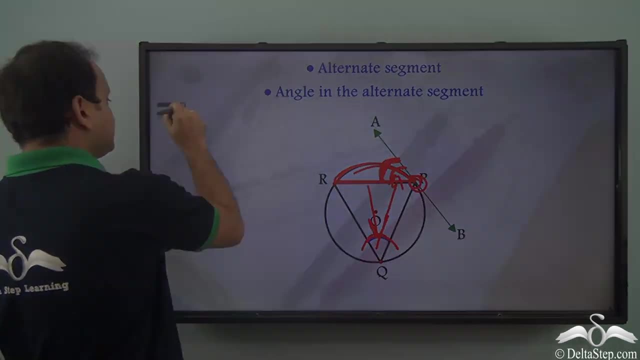 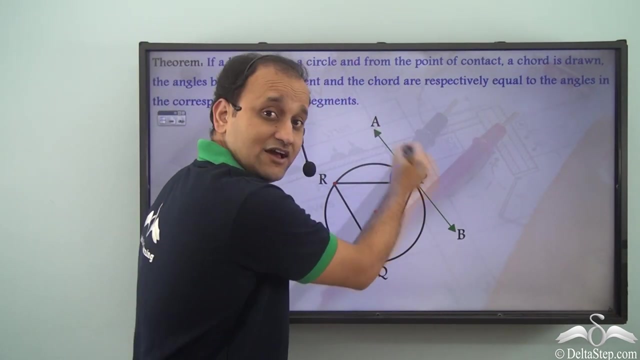 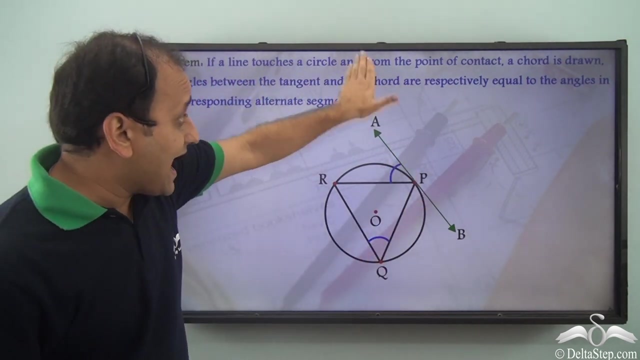 while the angle in the alternate segment has a special relationship with this particular angle. So let's discuss that. So the theorem states that if a line touches a circle, a line touches a circle. we have line AB which touches the circle at P. So if a line touches a circle and from the point of contact from, 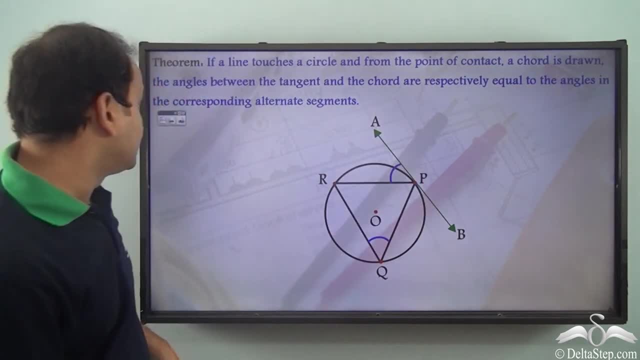 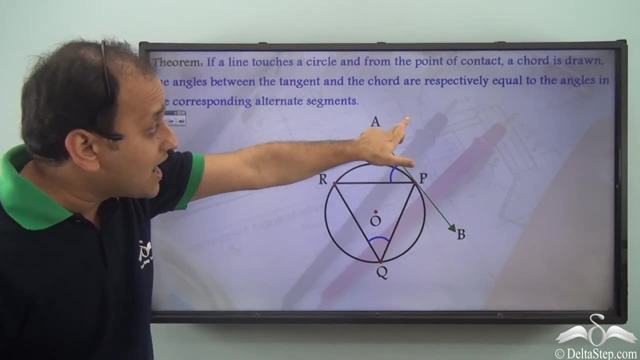 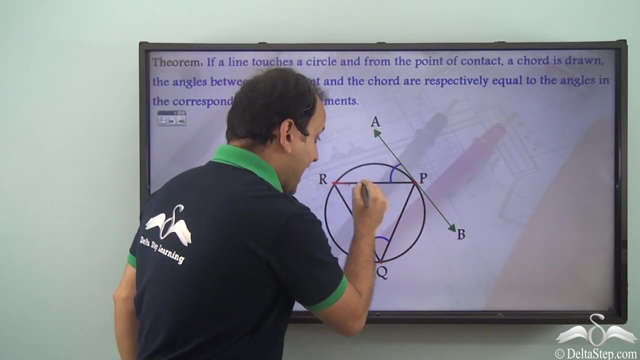 the point of contact P a chord is drawn, chord RP. the angles between the tangent and the chord are respectively equal to. So we are talking about angles between the tangent and the chord. The tangent is making angles with the chord, Basically two angles. 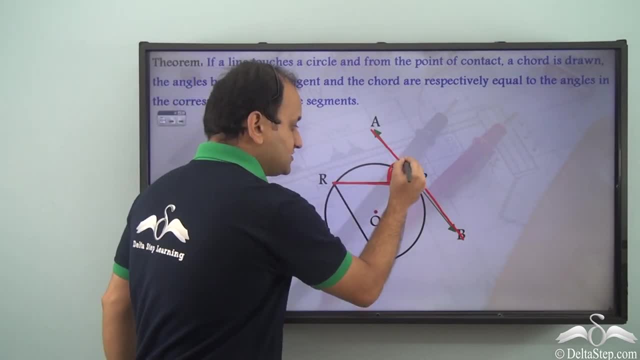 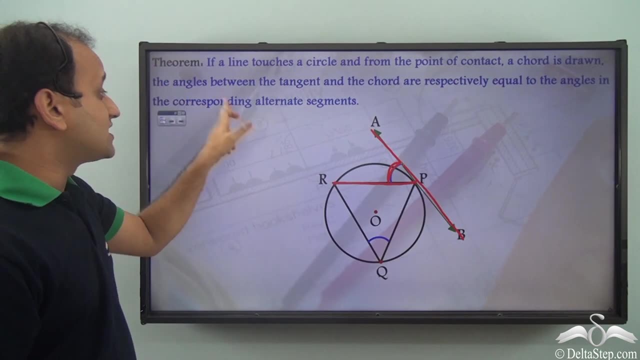 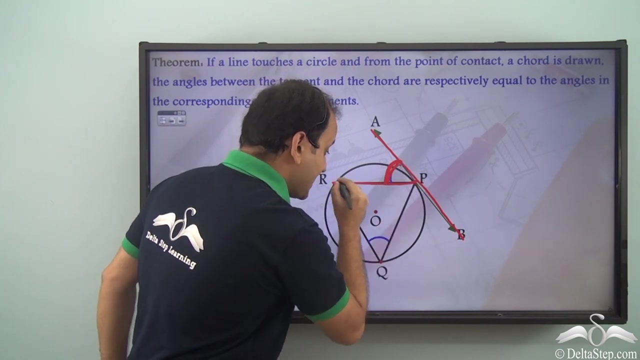 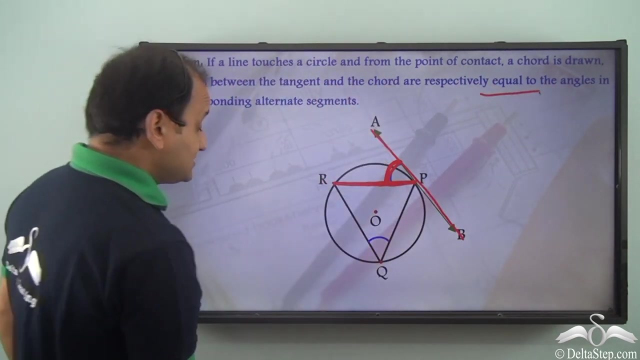 with the chord. So if we consider this angle first, so the angles between the tangent and the chord are respectively equal to the angles in the corresponding alternate segments. So angle made by the tangent and the chord is equal to the angles in the corresponding alternate 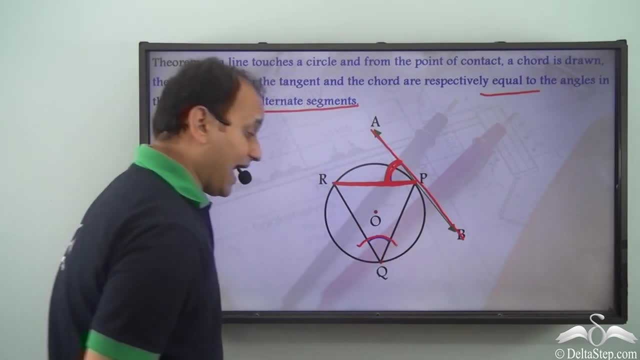 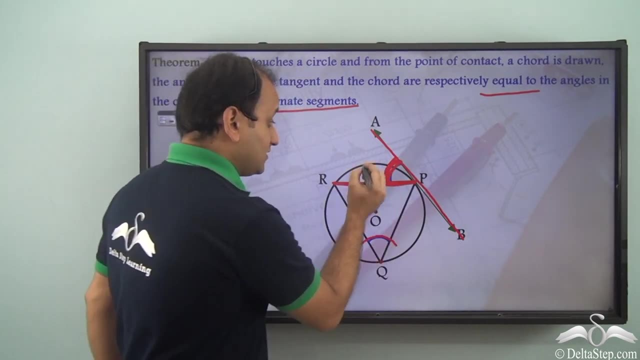 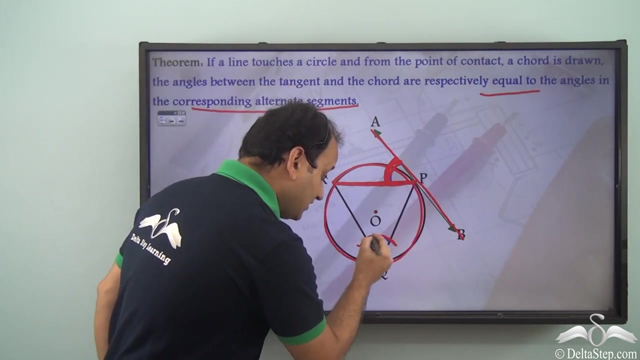 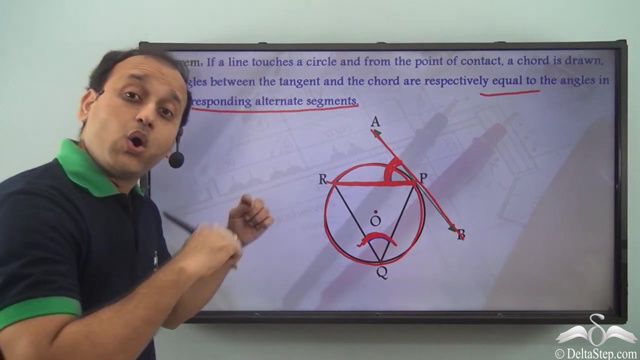 segments. Now, this is the angle in the alternate segment. If we are making an angle here, then it is touching this particular segment. What is the alternate segment? This is the alternate segment and this is the angle being formed by the same chord RP here in the alternate segment. So this angle will be equal to: 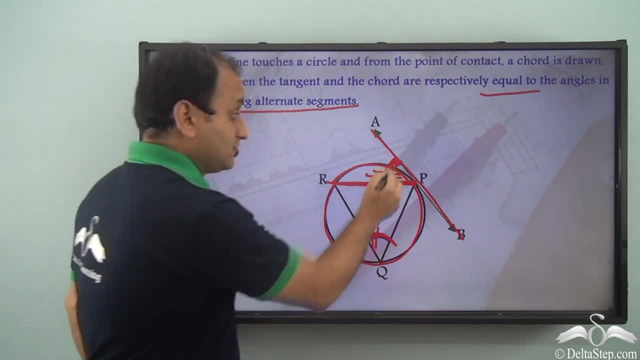 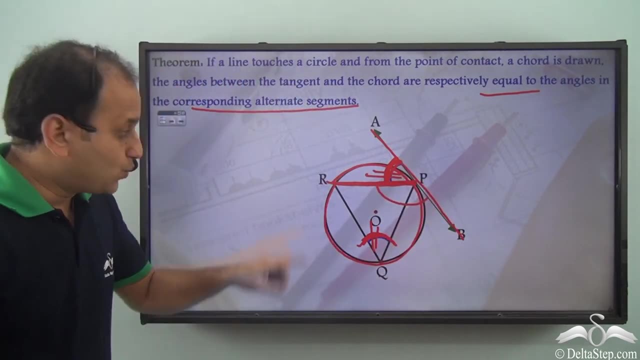 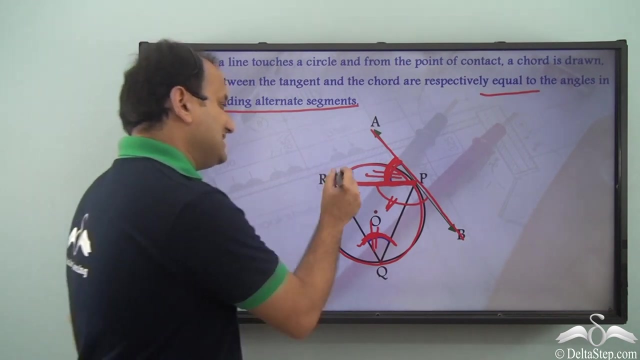 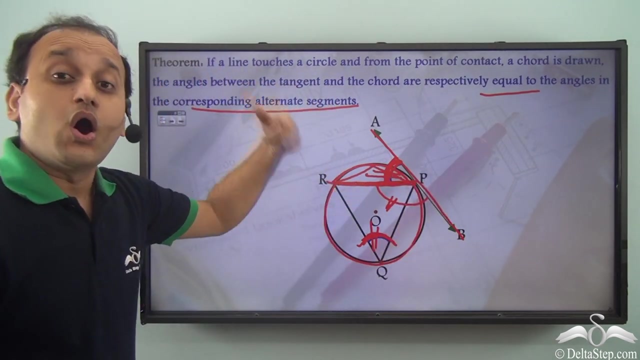 this angle. Similarly, this same tangent is also making an angle like this with the same chord. Now, what will this angle be equal to? Well, this angle will be equal to an angle formed by the same chord in the alternate segment. So when we are talking, 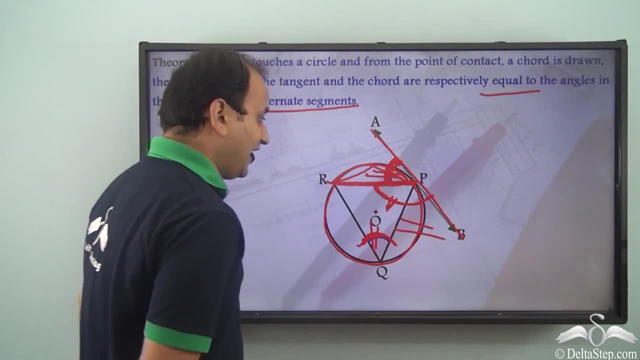 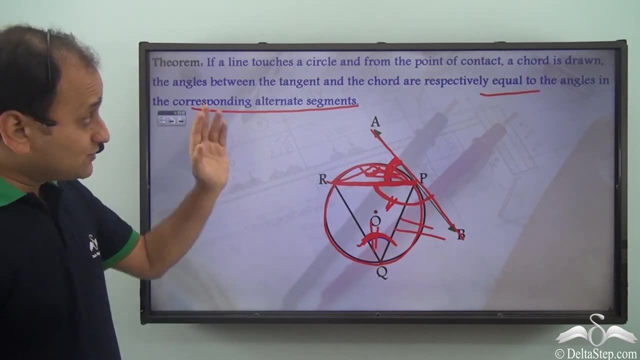 about this particular angle. it touches this segment, right? So we are talking about the alternate segment. So angle formed here by the same chord. So that's what this theorem states. If a line touches a circle, and from the point of 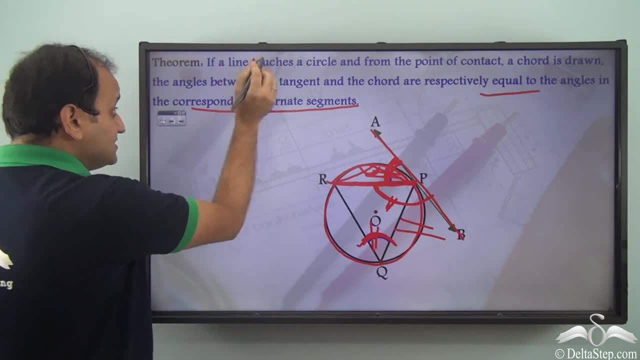 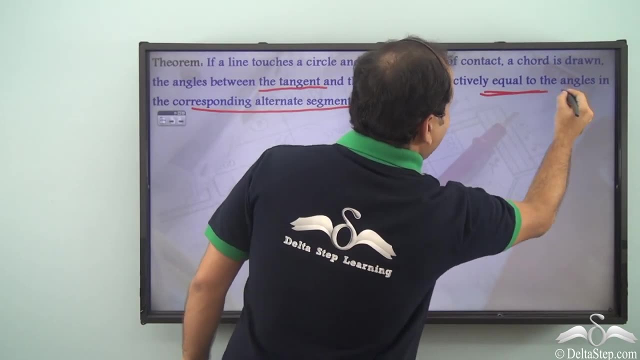 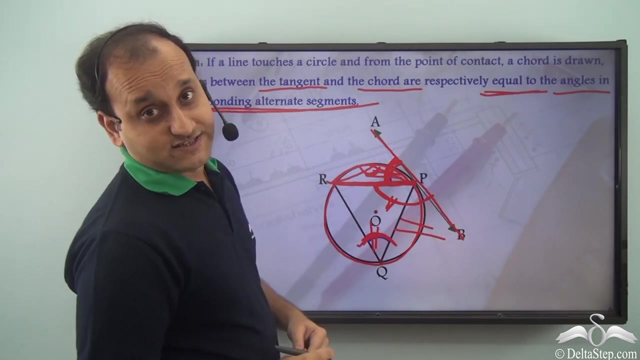 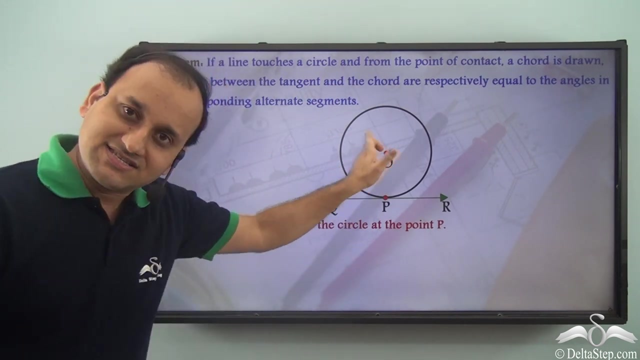 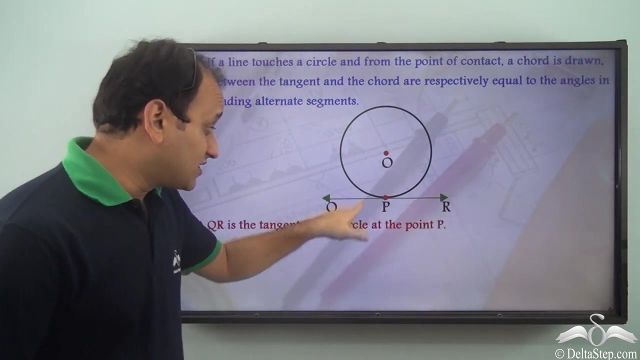 contact a chord is drawn, then the angles between the tangent and the and the chord are respectively equal to the angles in corresponding alternate segments. So let's see if we can prove this. So for that we have this particular circle whose center is O. Now we have this line QR which touches the circle at P, So we can say that 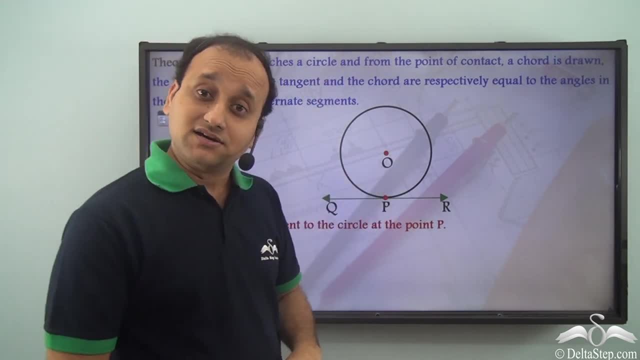 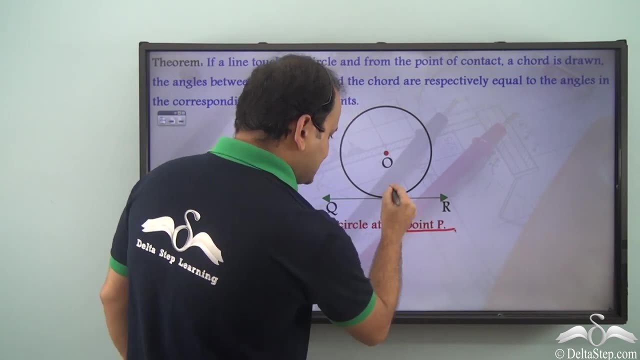 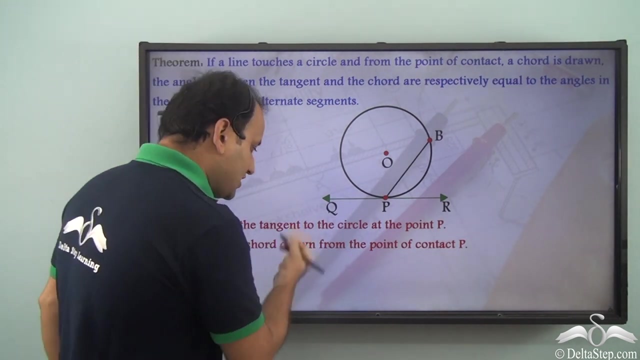 QR is a tangent to this particular circle. So what is given? First of all, QR is the tangent to the circle at point P. Now, second is that PB is a chord drawn from the point of contact P. So we have a chord PB which is drawn from. 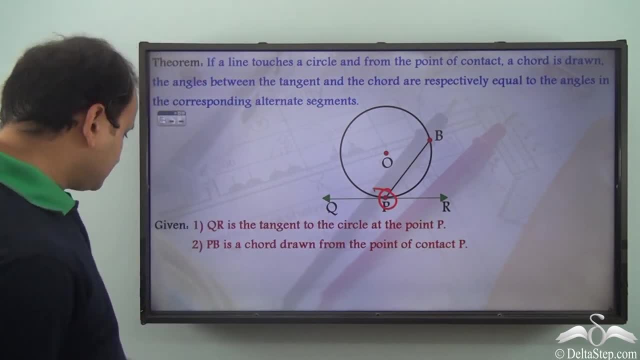 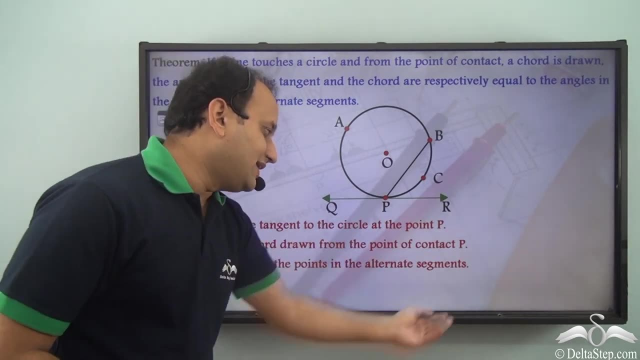 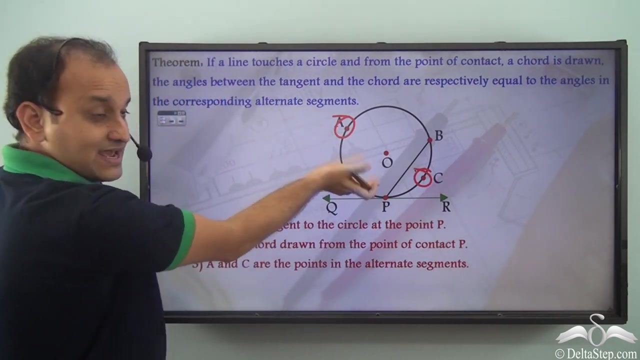 the point of contact of this particular tangent. And third, our cube, therefore, is a tangent to the circle at O, because this particular third thing which is given is that A and C are the points in the alternate segments. So we have this point here and this point here. Now both lie in alternate segments. 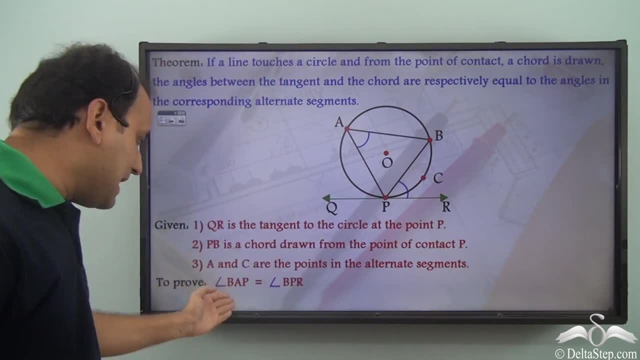 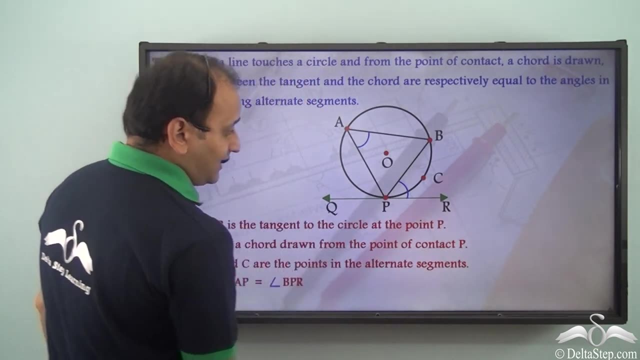 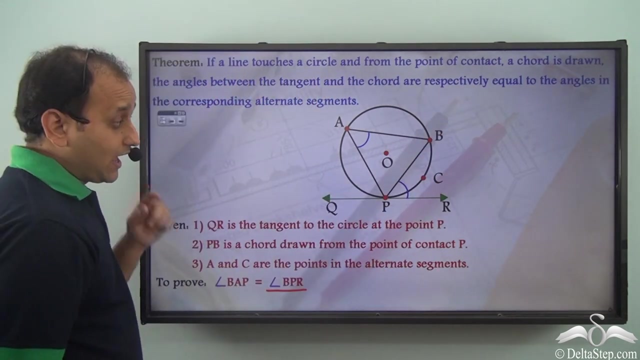 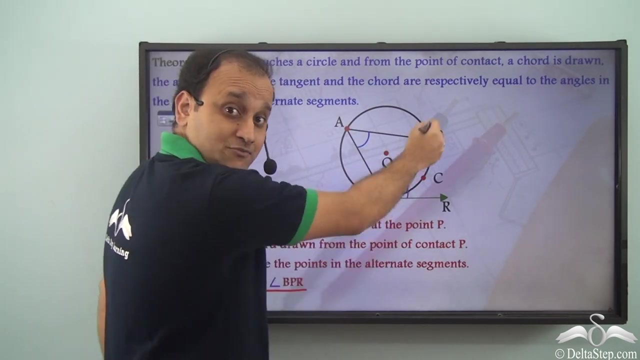 Now what we need to prove. We need to prove that angle BAP is equal to angle BPR. As you can see clearly, this tangent QR is making an angle BPR with this chord PB. Now the theorem states that this angle should be equal to the angle made by the same chord in the alternate. 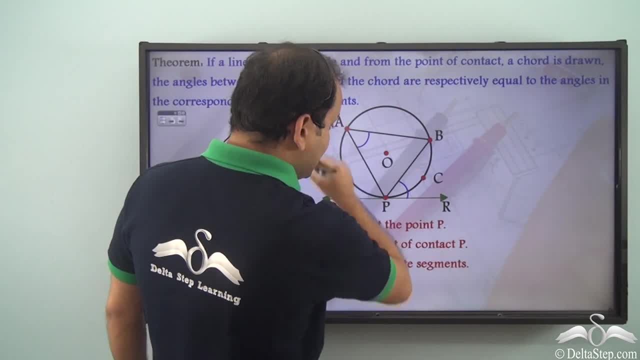 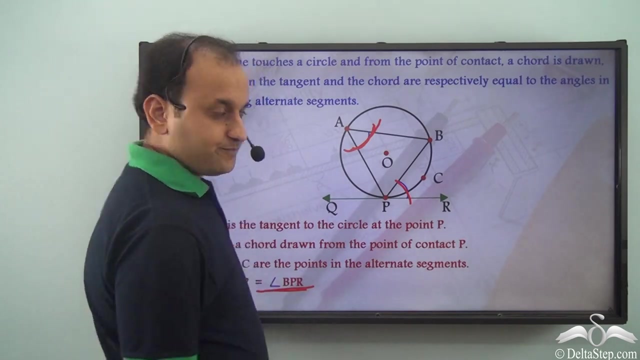 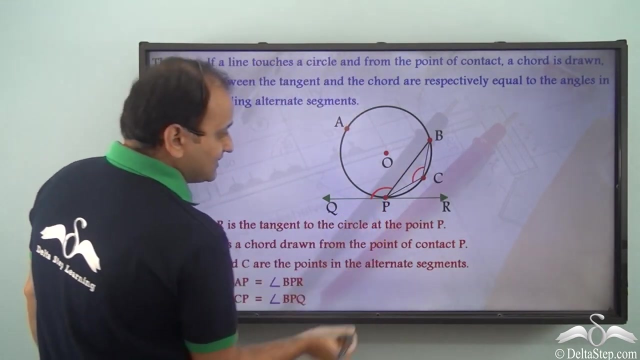 segment. So this is the alternate segment, PAB. So this angle made here is the angle made in the alternate segment. So this angle should be equal to this angle. That is, angle BAP should be equal to angle BPR. That's what we need to prove. Also, angle BCP is equal to angle BPQ. Now you can see. 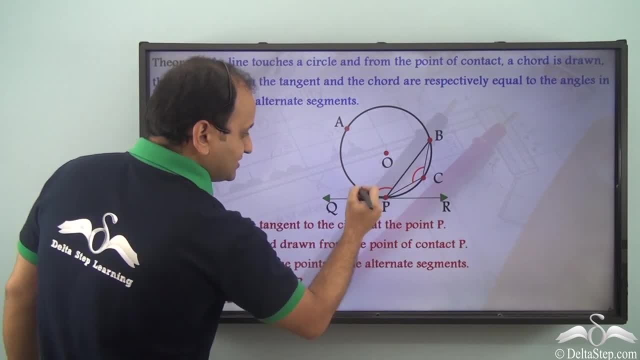 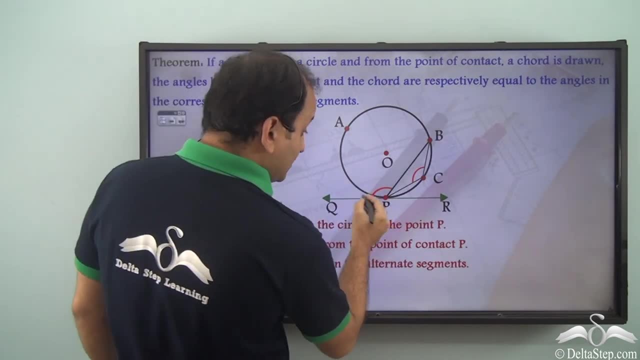 that the same tangent is also making this particular angle here, angle BPQ with the same chord PB, But now the segment has changed. If we talk about this particular angle here, then we can see that the segment has changed. Now, if we talk about this particular angle here, then we can see that the segment has changed. 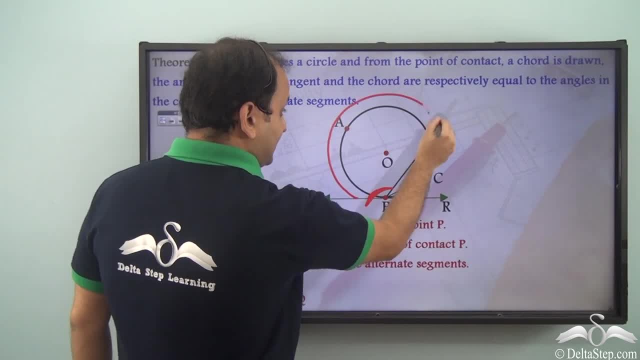 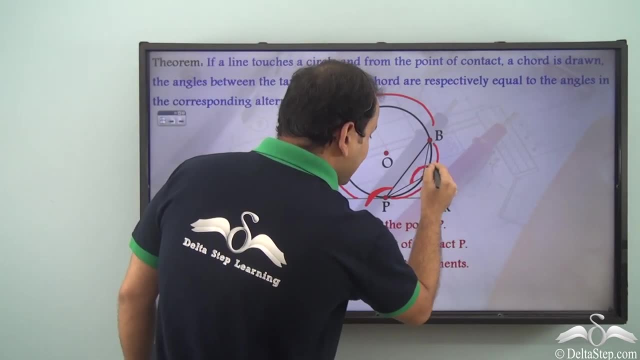 In this particular case, if this angle is made a certain angle, then this is touching this particular segment. So what is the alternate segment in this case? This is the alternate segment and angle made in the alternate segment is this by the same chord, PB, So this angle. 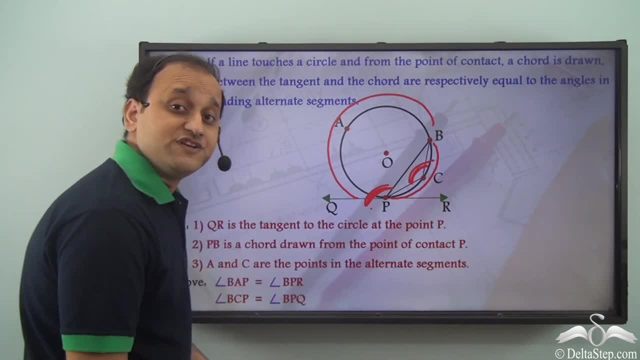 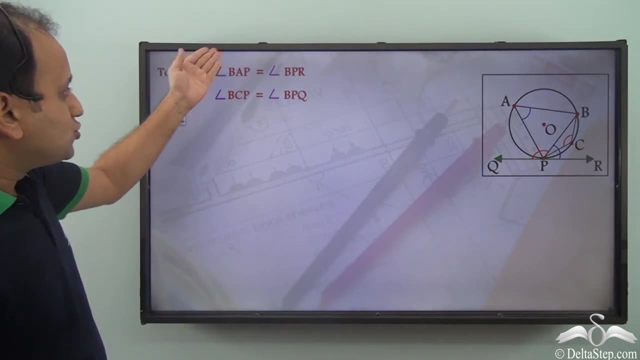 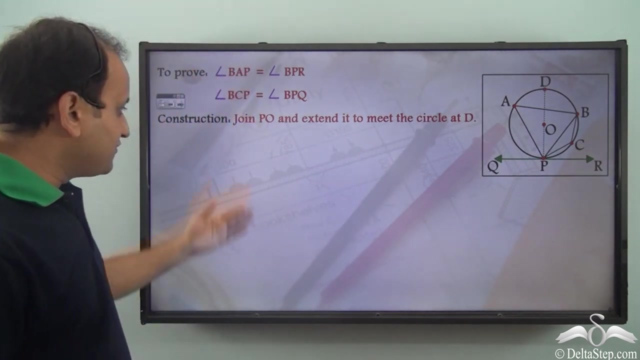 will be equal to this angle. This is another point which we need to prove, So let's start with the proof. So these are the two things which we need to prove, And for that this, we need to perform a construction. So what we do is: 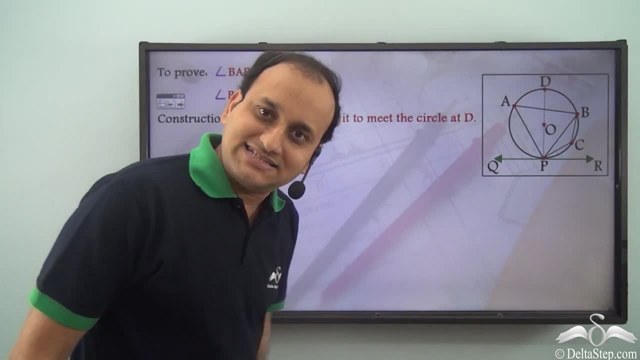 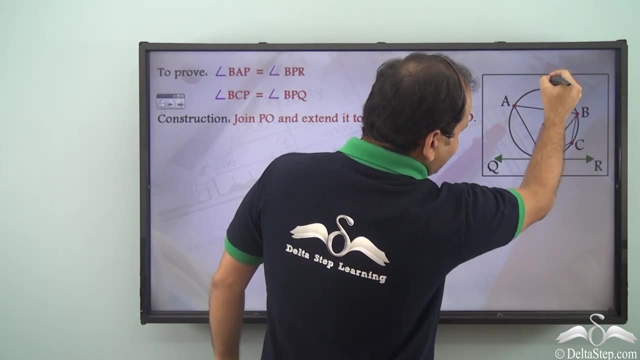 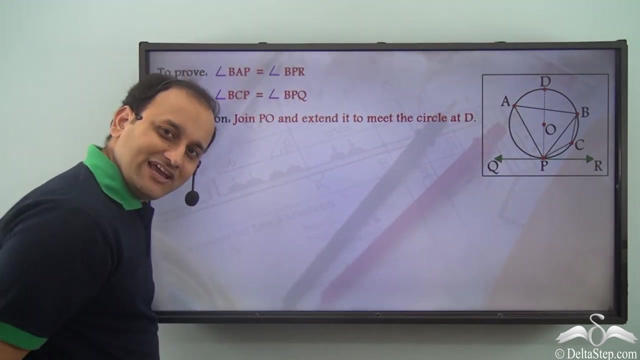 we join PO and extend it to meet the circle at D. So we join PO, O, which is the center of the circle, and we extend this till D. That is again a point on the circle. So what do we get here? We get: 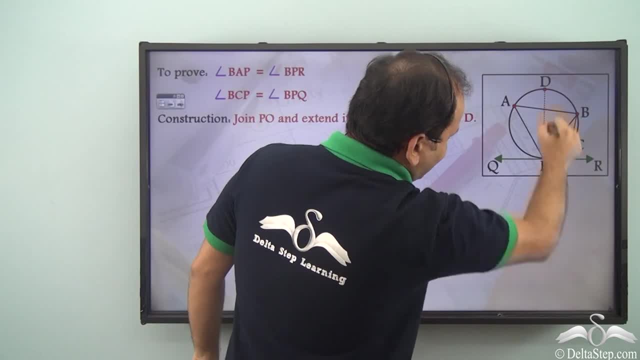 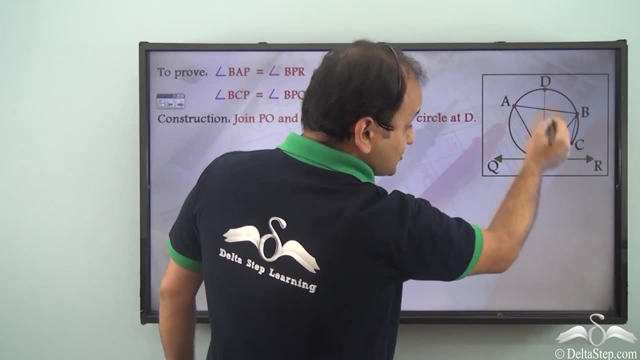 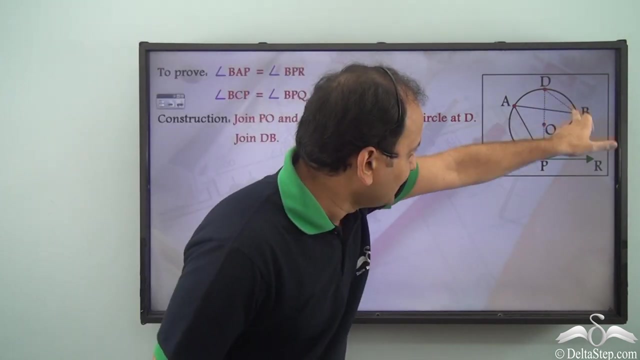 diameter of the circle. We can say that PD is nothing but diameter of the circle, because it is passing through the center and joins two points on the circle. Now we also join DB. We also join DB these two points on the circle. So first of all, 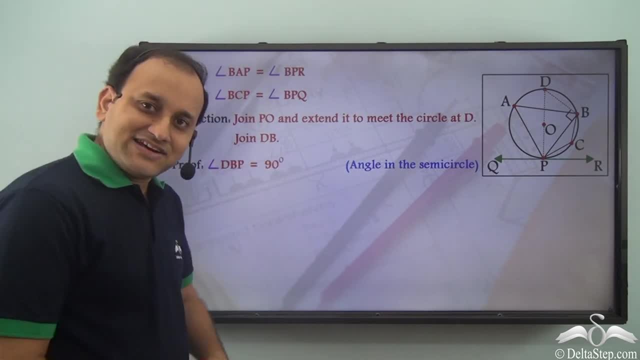 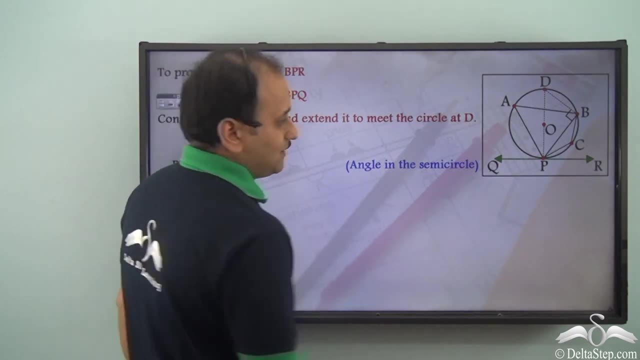 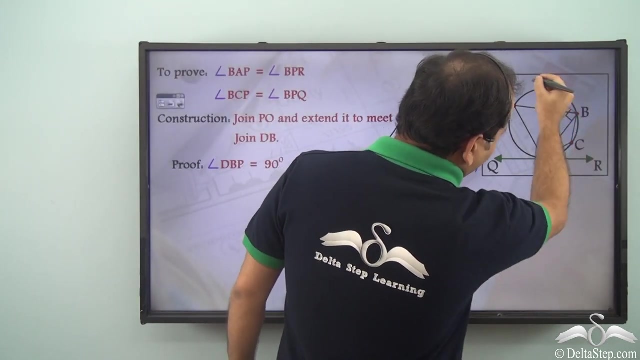 we can say that angle DBP is equal to 90 degrees. Why do I say so? Because angle DBP is nothing but angle in a semicircle, because DP is a diameter of the particular circle and it is making an angle here. So this will be 90 degrees because it is. 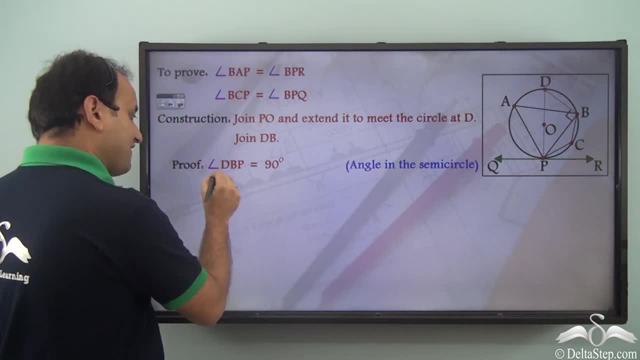 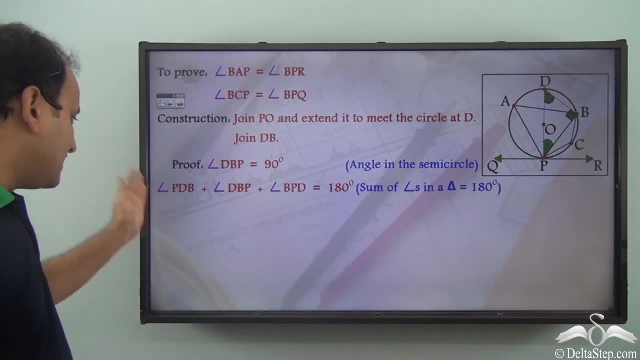 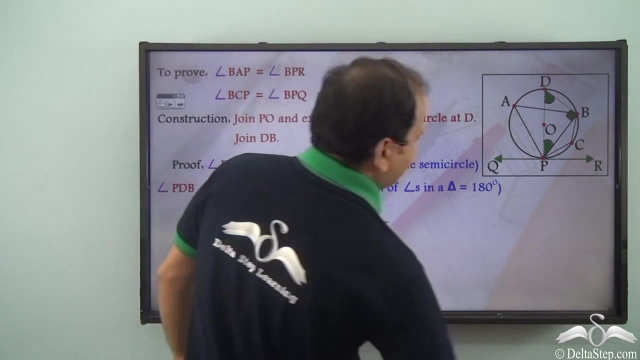 an angle in the semicircle. So we have angle DBP is equal to 90 degrees. Next we can say that angle PDB plus angle DBP plus angle BPD. So we are talking about angle PDB, angle PDB, this angle plus angle DBP. 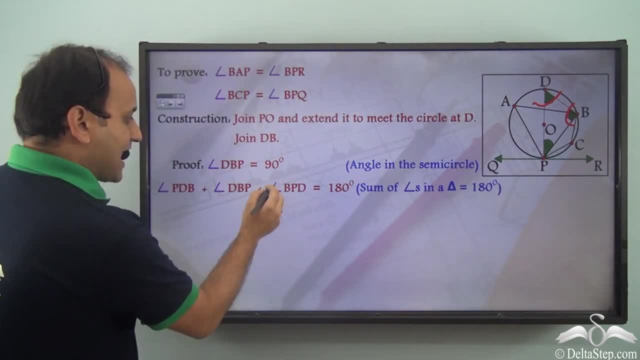 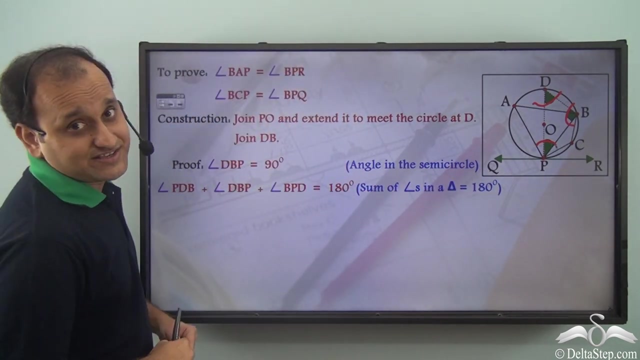 angle DBP and angle BPD. angle BPD, this angle. If we add these three angles, it will be 180 degrees, because sum of angles in a triangle is always 180 degrees. So we get this particular equation here. Now, what do we know about angle DBP? 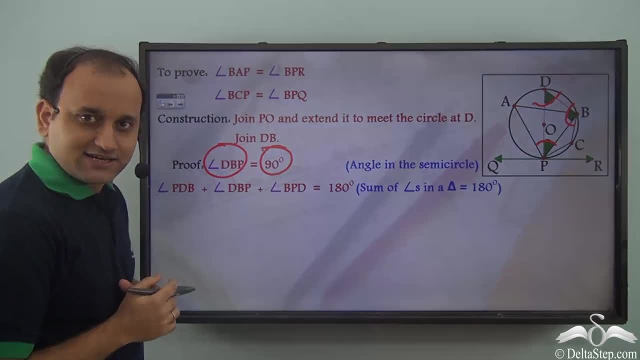 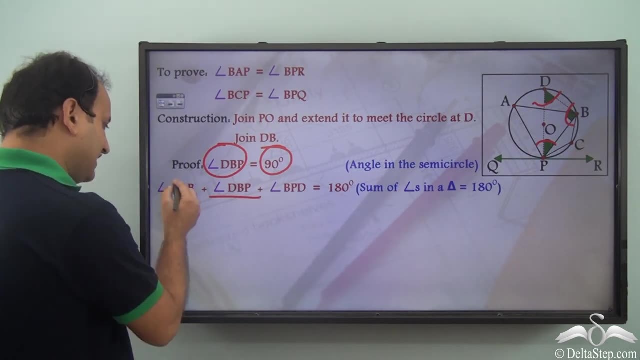 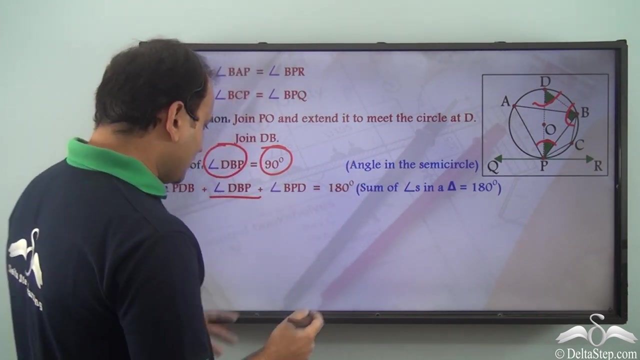 Its value is 90 degrees, isn't it? Now, if we substitute this value here, then what do we get? We get angle PDB plus 90 degrees plus angle BPD is equal to 180 degrees. So if 90 degrees comes this side, then it will be 180 degrees. 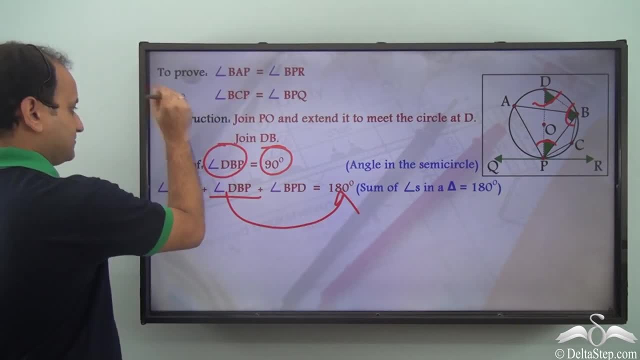 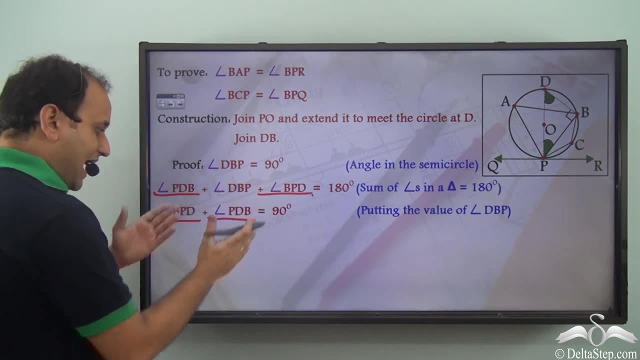 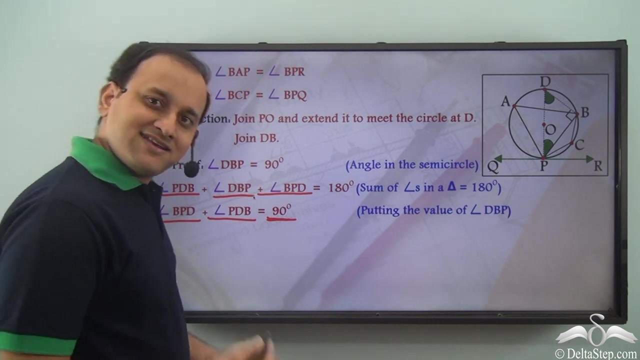 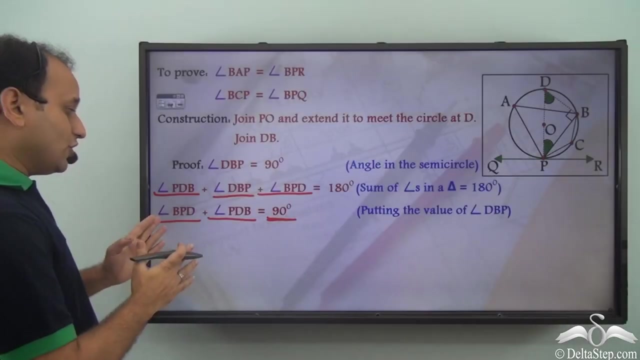 minus 90 degrees. So what do we get from that? We get angle BPD plus angle PDB plus angle DBP db. that is, these two angles added will give us 90 degrees, because 180 degrees minus angle dbp is 90 degrees. So angle bpd plus angle pdb is equal to 90 degrees. So this is one. 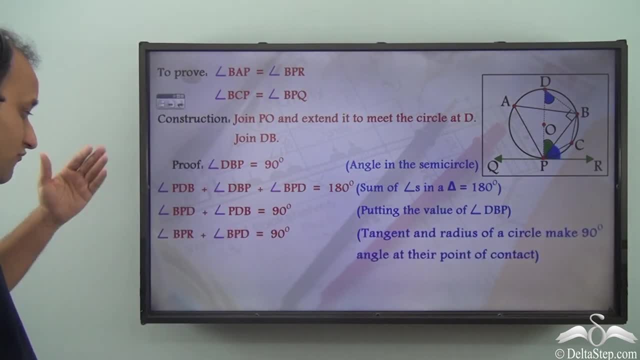 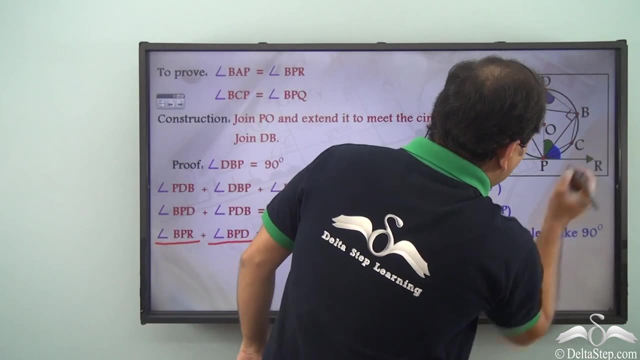 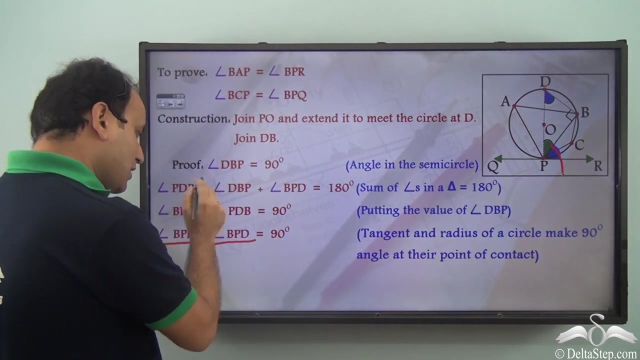 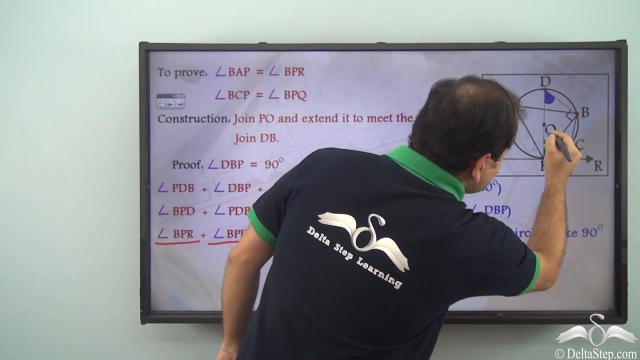 point. Now we can also say that angle bpr plus angle bpd is equal to 90 degrees. Let's see, we have angle bpr. We are talking about this particular angle, This plus angle bpd, Angle bpd. So we are talking about this particular angle here. Now, if we add both of them, we 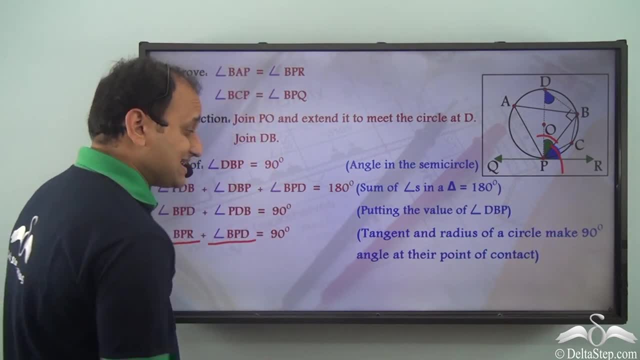 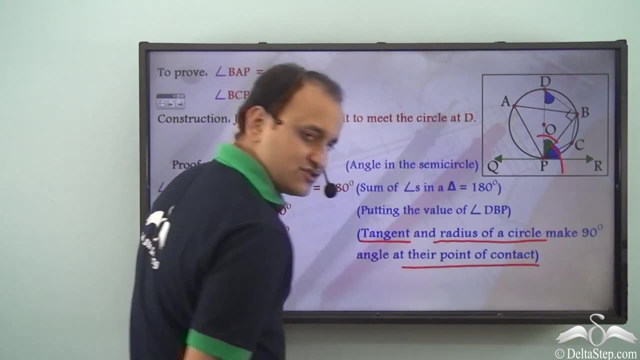 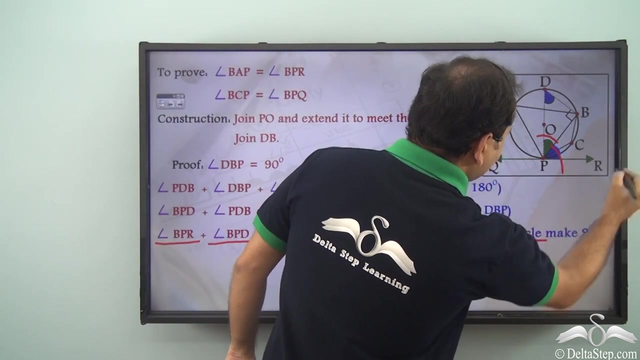 get 90 degrees. Why do I say so? Because tangent and radius of a circle make 90 degree angle at their point of the circle of contact, isn't it? We know about this particular theorem, That is, we have this particular tangent and OP is nothing but radius of this particular circle. So 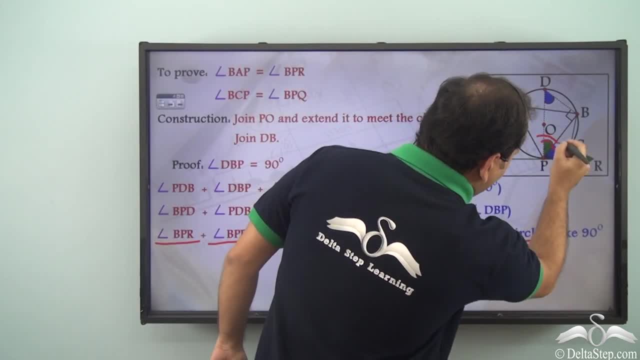 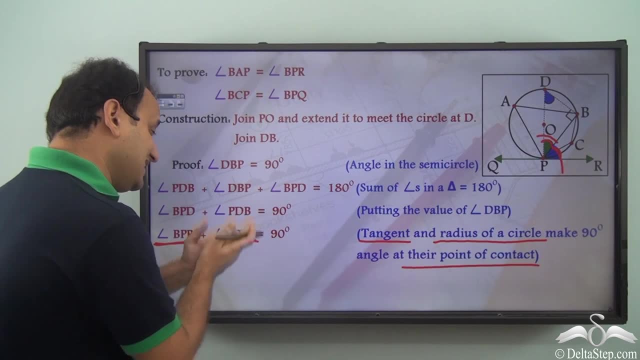 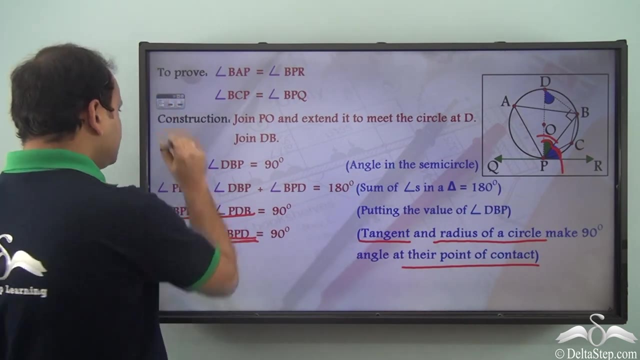 both of them will make 90 degree angle. So these two angles will add up to 90 degrees. So angle BPR plus angle BPD will be equal to 90 degrees. Now, from these two equations, what can we derive? We can say that angle BPD plus angle PDB will. 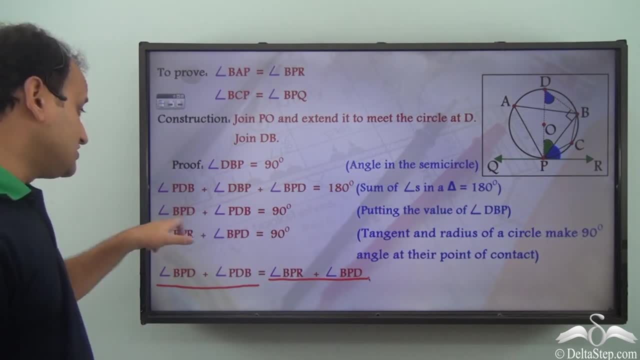 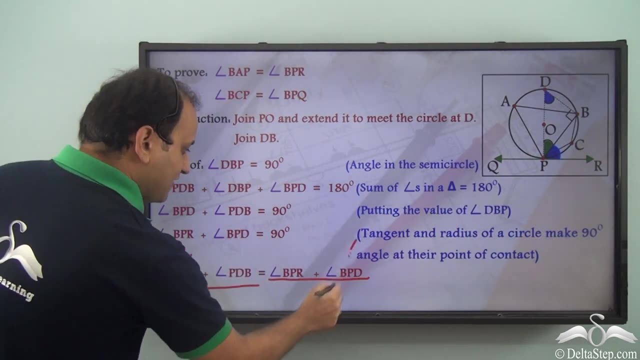 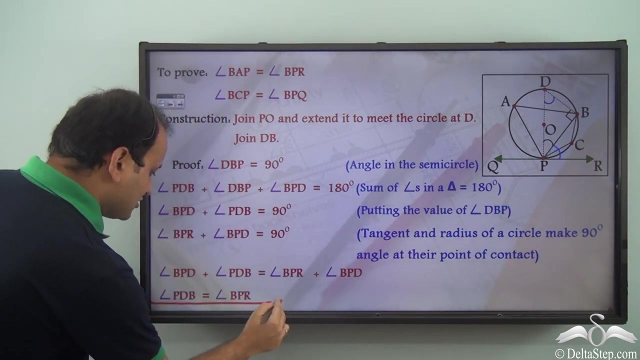 be equal to angle BPR plus angle BPD, because both of them add up to 90 degrees. Now again, in this case we have BPD which can cancel out. So what is left? Angle PDB is equal to angle BPR, So we were able to. 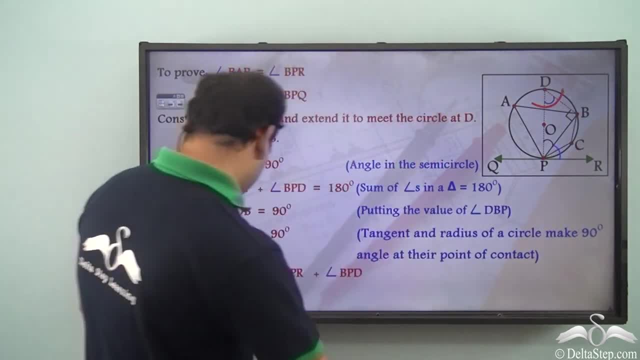 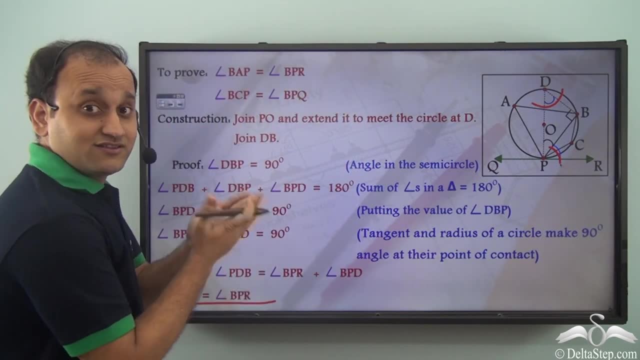 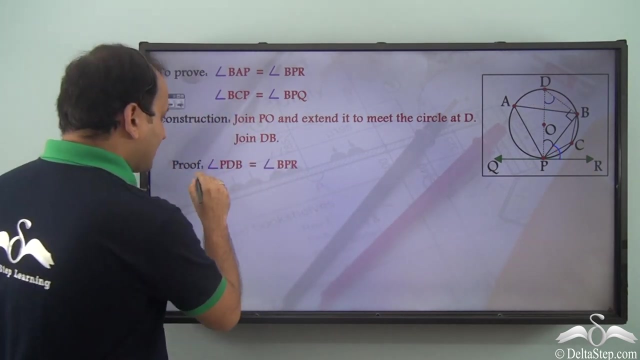 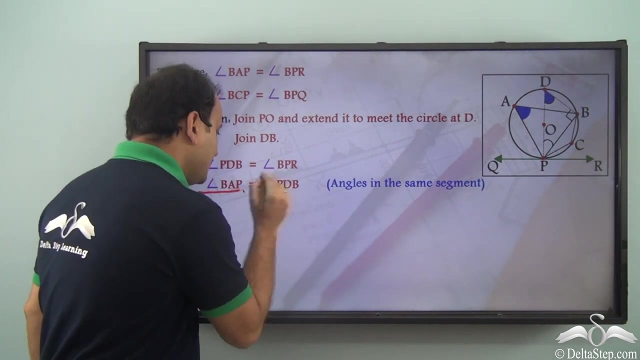 prove: angle PDB is equal to angle BPR. this angle, But this is not the final thing which we need, So we need to go further. So this is our current finding. From this, we can also say that angle BAP is equal to angle PDB. Why do I say so? 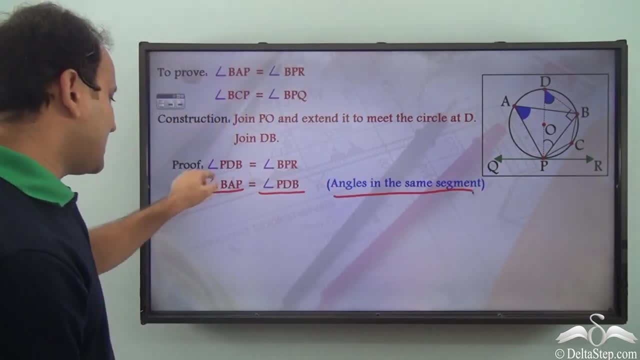 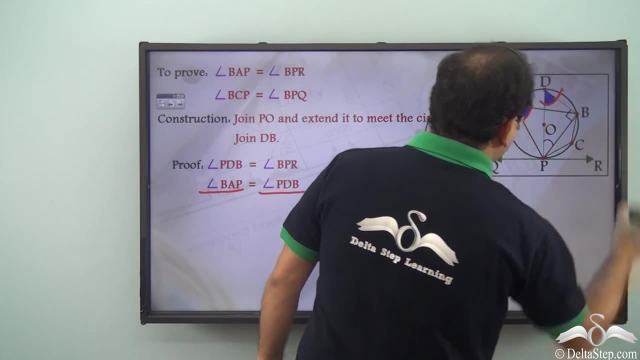 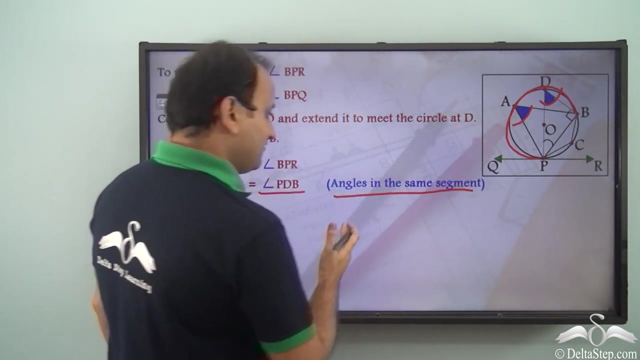 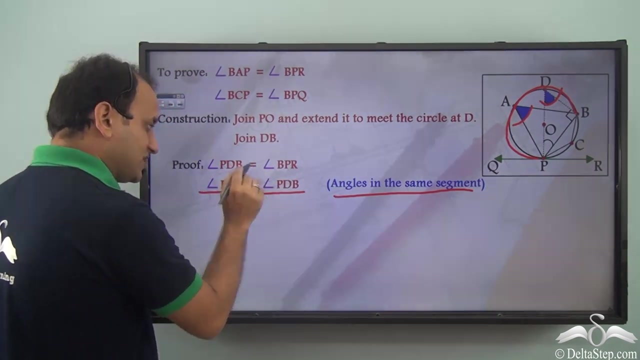 Because they are in the same segment: Angle BAP- this angle- and angle PDB- this particular angle. both lie in the same segment, isn't it? And that's why they will be equal, So their values will be same. Now again, we have two equations. Angle PDB is equal to. 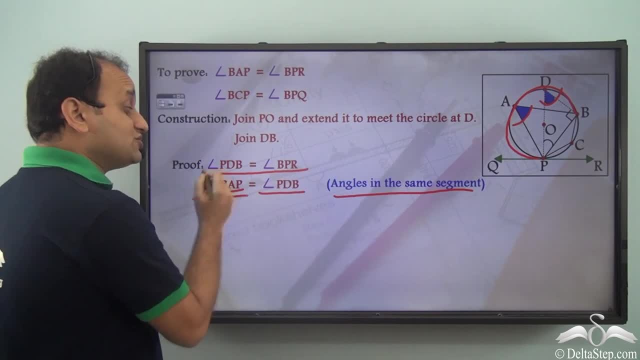 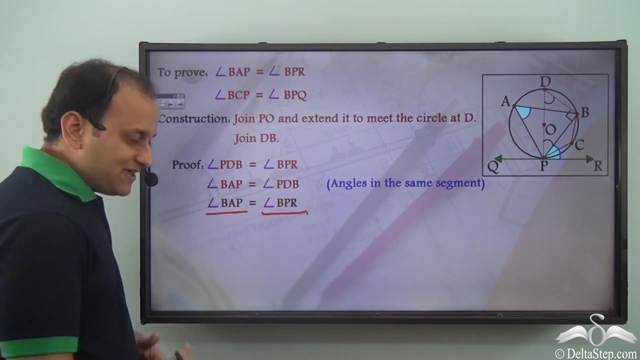 angle BPR and angle BAP is also equal to angle PDB, So both these are equal to angle PDB. So from this we can say that angle BAP is equal to angle BPR, because both of them are equal to angle PDB. So they both are equal too, and that's what. 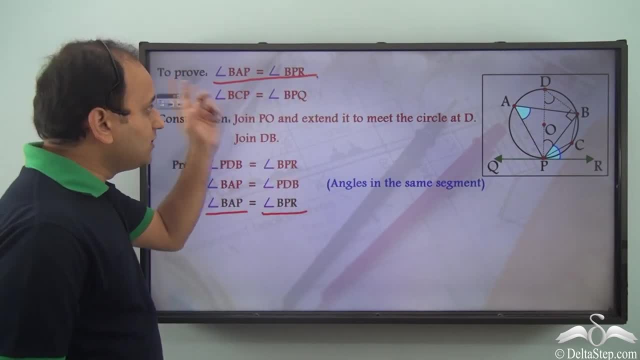 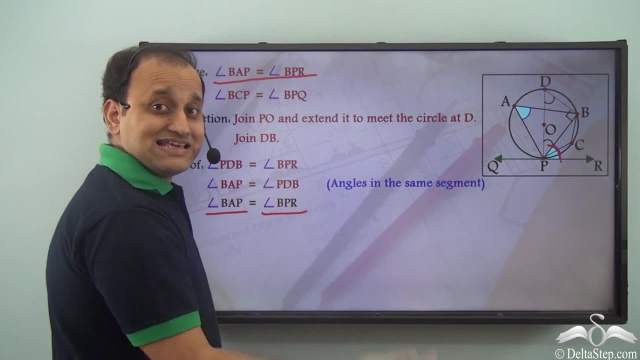 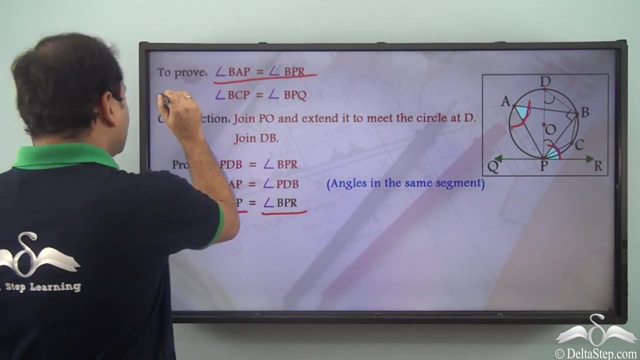 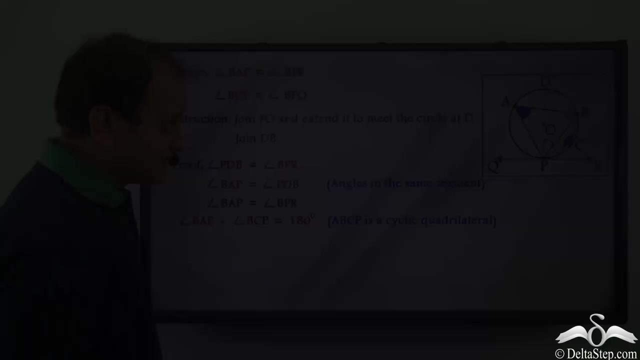 we needed to prove. Angle BAP is equal to angle BPR. That is, this angle made by the tangent with the chord is equal to the angle in the alternate segment. Now we can also say that angle BAP plus angle BCP equal to 180 degrees Angle BAP, this particular 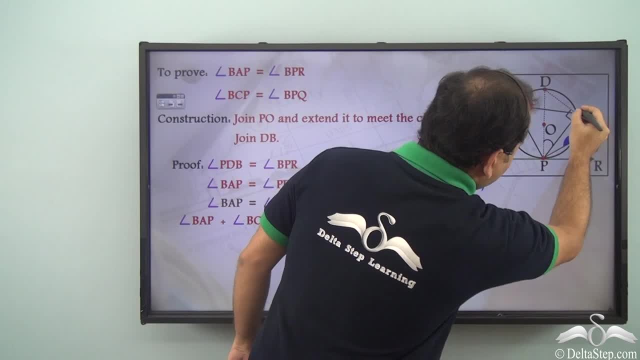 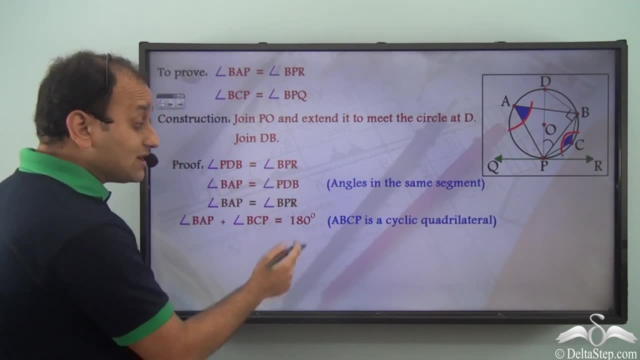 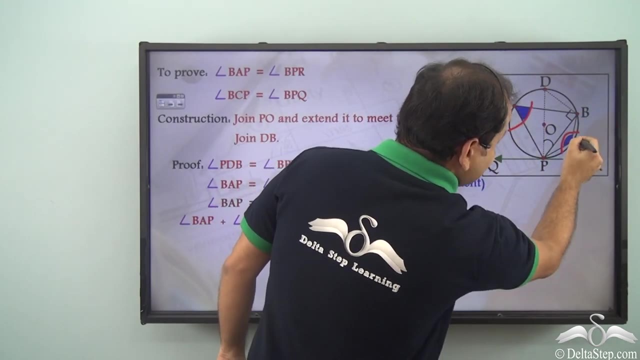 angle plus angle BCP. Angle BCP is equal to angle BAP. This particular angle, both will add up to 180 degrees. Why do I say so? Because ABCP is a cyclic quadrilateral. If you notice A, B, C and P, all the four points. 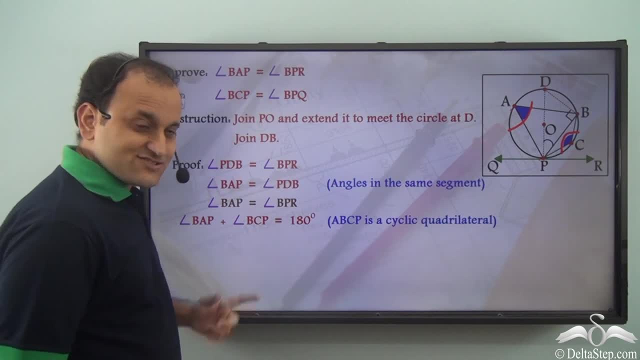 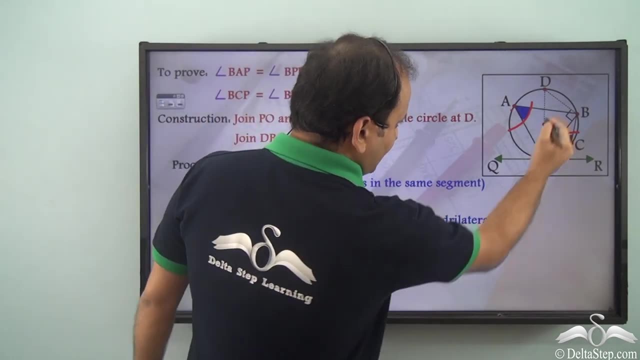 lie on this particular circle. That is, all the four vertices of this particular quadrilateral lie on the same circle, And so this is a cyclic quadrilateral. Taking some numbers, let us assume that A in the right figure is equal to 180 and一點. 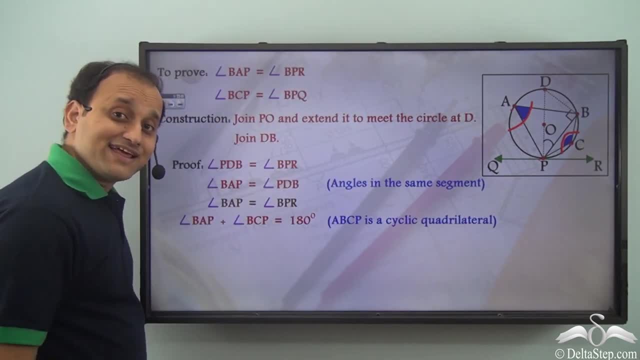 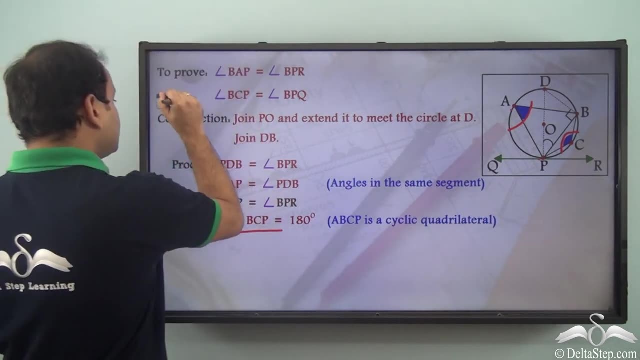 and B in the left is 180 degrees. We know that angle BPR and Cathedral will add up to 180 degrees, So using the same number of them, all will add up to 180.. So angle BAP plus angle BCP is equal to 180 degrees. Now you also know that angle BPR plus angle BPQ. 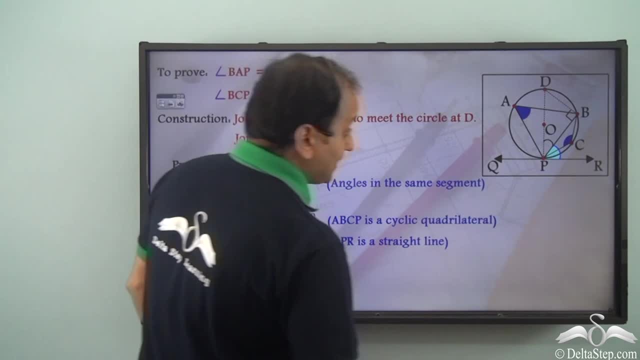 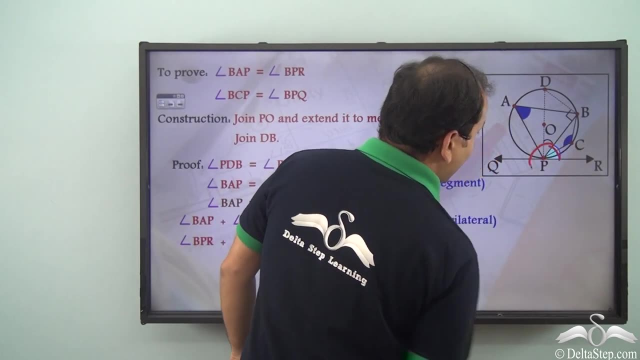 will be 180 degrees. It's very simple, Because BPR is this particular angle and BPQ is this particular angle. As both of them together, there will be f of fит, which will be 그렇죠, Both are equal, and it will always add up to f of tabs rechts and either best to the. 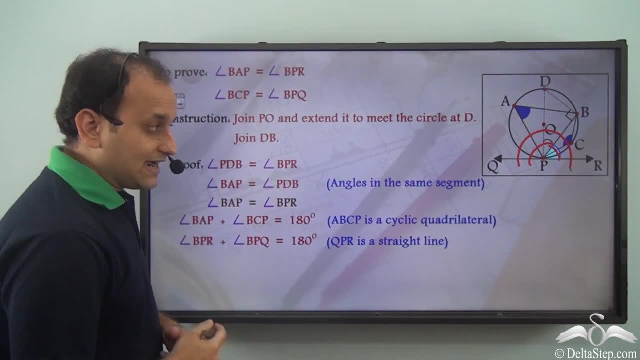 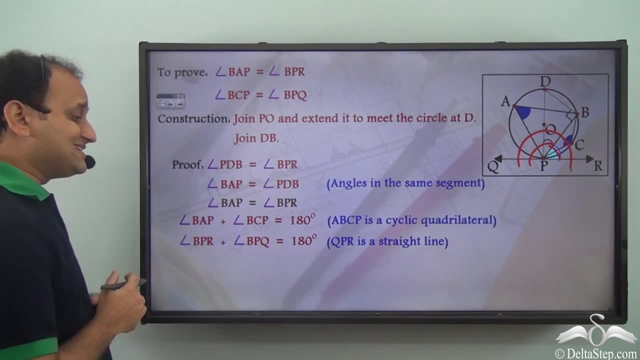 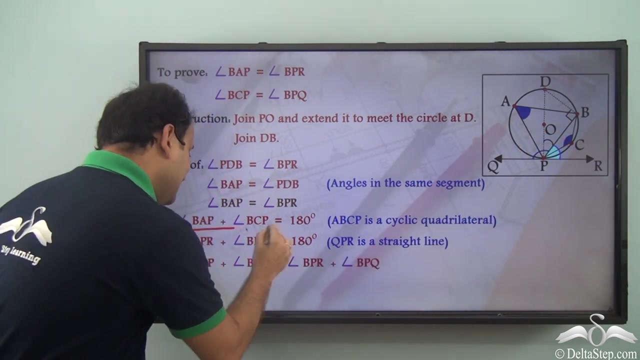 left or the right when trying to measure love curve of the ended angle, make a straight angle that is 180 degrees. So angle BPR plus angle BPQ will also be equal to 180 degrees. Now what do we derive from that? That this: 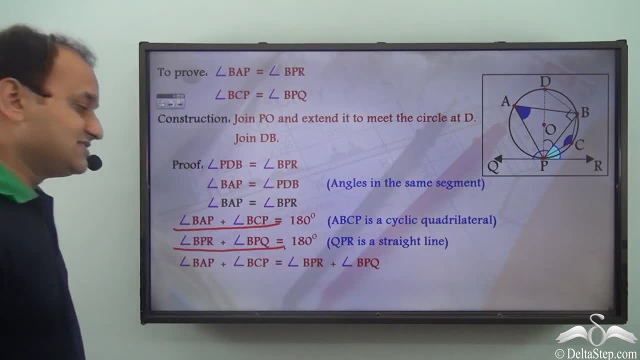 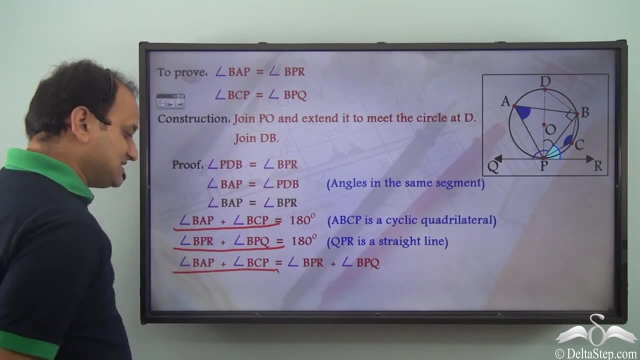 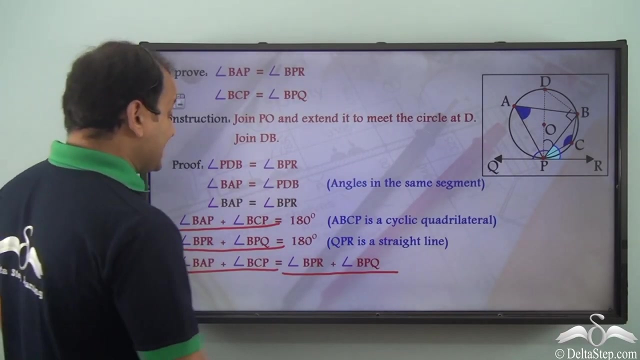 is equal to 180 degrees, and even this is equal to 180 degrees, So they both are equal. So angle BAP plus angle BCP is equal to angle BPR plus angle BPQ. Now we know that angle BAP is equal to angle BPR. 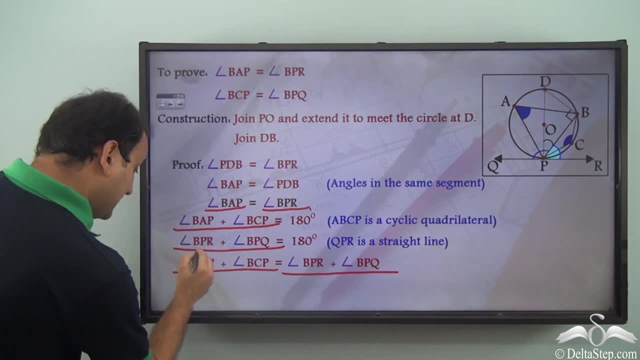 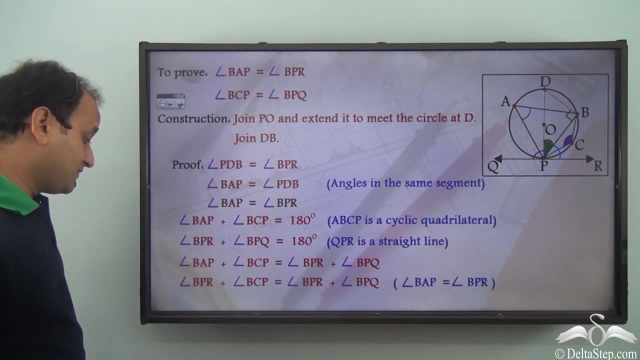 We have already proved that. So we can substitute one of the angles with the other. So we can write angle BPR, which is basically we have just replaced angle BAP with BPR, because both of them are equal. So angle BPR plus angle BCP is equal to. 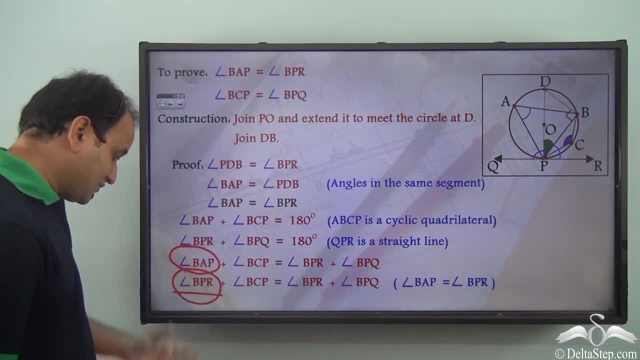 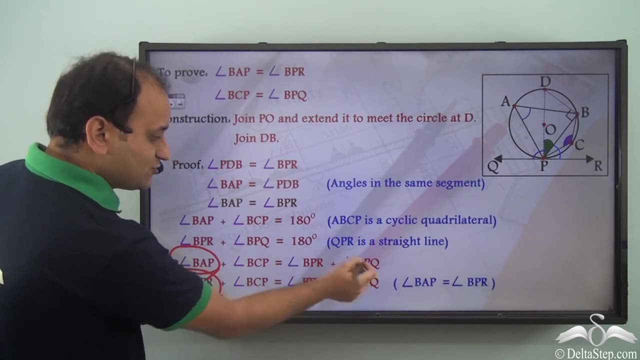 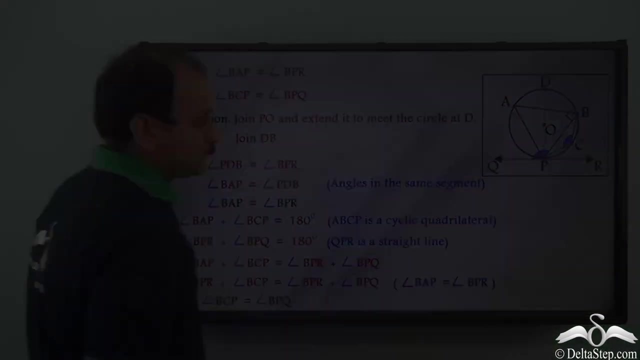 angle BPR plus angle BPQ. So now we have BPR on both the sides, We can cancel them out, and what have we got? Angle BCP is equal to angle BPQ, So angle BCP is equal to angle BPQ. Angle BCP is equal to. 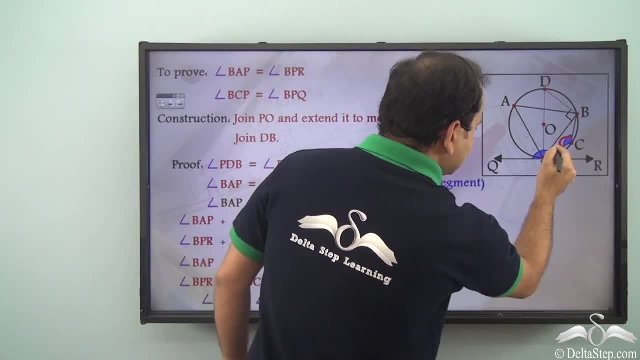 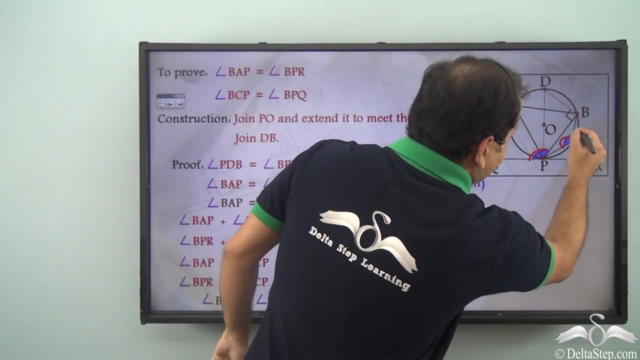 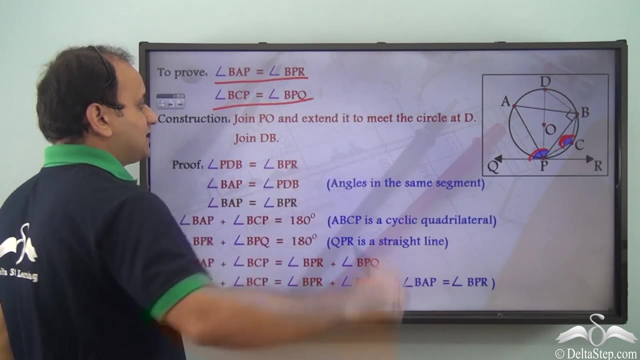 angle BPQ. This particular angle, that is, angle made by the tangent with the chord, is equal to the angle in the alternate segment. So we have proved this too. So we have proved both of them, and which means that the theorem which we had discussed-